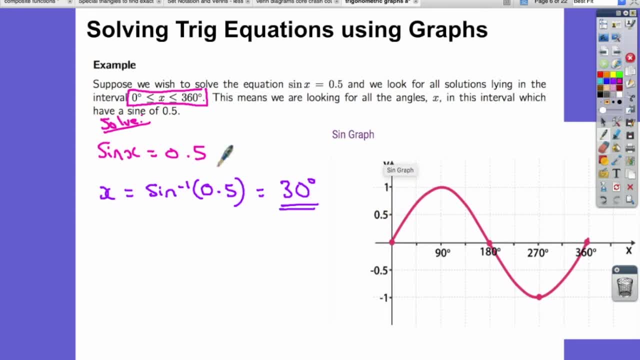 OK, now let's go and have a look. Now we know that the answer we're after when we put x in is 0.5.. So if we actually go across from the 0.5 and read down, you can see it looks about right. 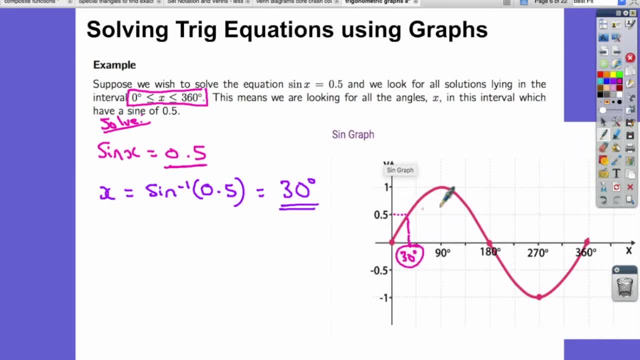 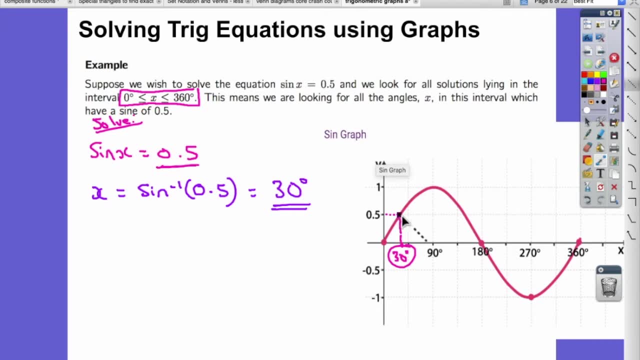 doesn't it? OK, there's 30 degrees, But there's another answer in this particular domain. OK, and we get that by continuing that straight line across And we're going to hit the graph again at the next answer. And the next answer looks like it's just before. 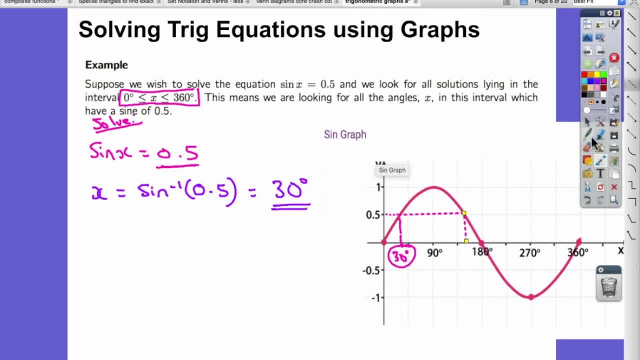 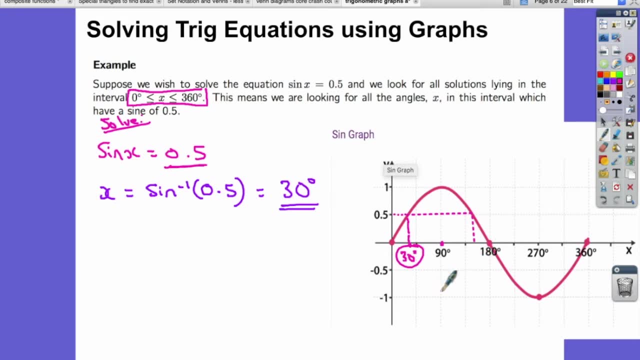 190 degrees And we can also see that this peak here. All right, It's completely symmetrical with 90 in the middle, All right. So hopefully you could use the idea of symmetry to actually find what this next answer would be. 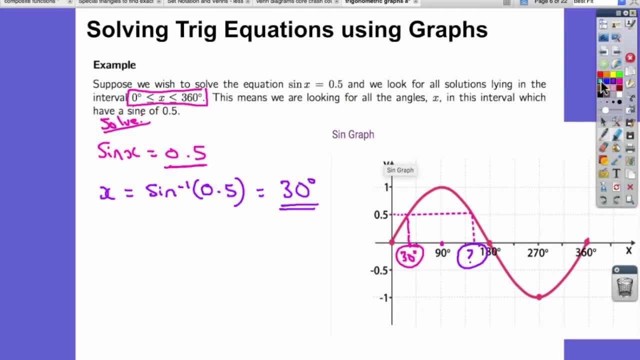 All right Now. the way that I usually do it is, I think: well, this difference here, going from 0 to 30, is 30. So it must match on this side. OK, so I hope you agree that my next answer here. 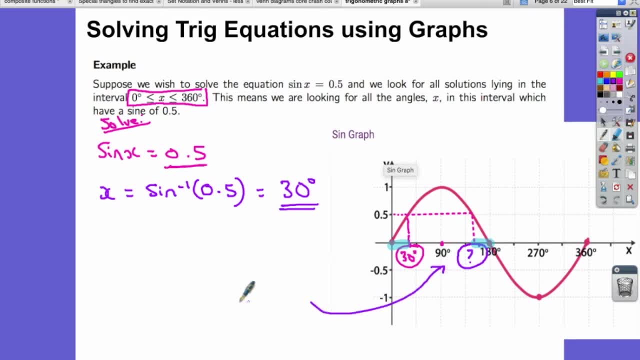 is actually going to be 180 degrees subtract 30 degrees, which is 150 degrees. That's my second answer. All right, And I could also, you know, obviously I can go and check that, So I'm going to put that into my. 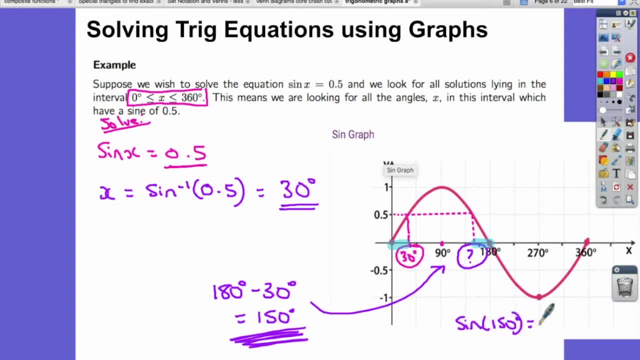 calculator now Sine 150 degrees equals. Yes, it does. It equals 0.5.. So you can go and check Now. I don't think there's definitely no more answers here, because then the graph is going below the x-axis to give negative values of sine x. 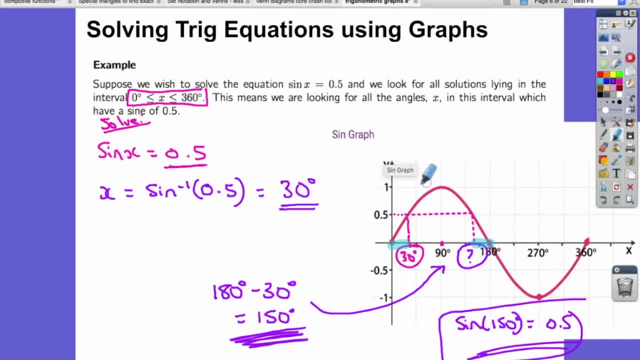 So they're my two answers. OK, so I've got two answers to the first question: 30 degrees and 150 degrees. OK, let's go and have a look at a cos x example. So here's the cos graph. OK, and again. 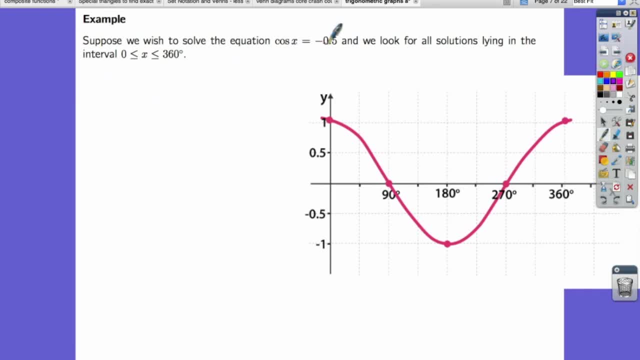 similar sort of question, very similar sounding. So it says cos x equals negative 0.5, looking at the same domain, So x line between 0 and 360 inclusive, And the first thing I'm going to do again is I'm going to do cos to the minus 1 of negative 0.5. 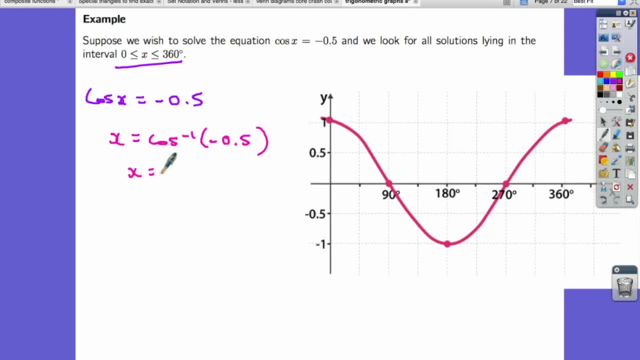 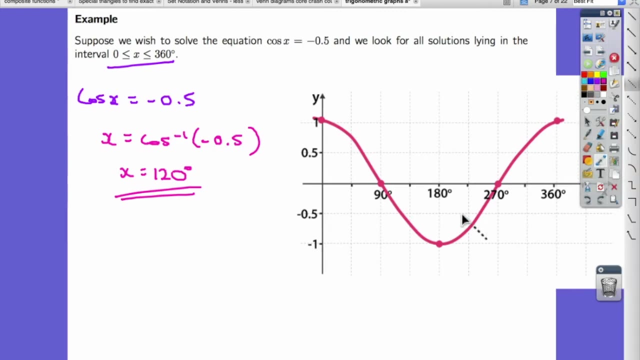 So that's going to give me an answer of 120 degrees. Now does that match up with what I can see on the graph? Let's double check. So let's go across from negative 0.5 and hit the graph. I want my straight line. Let's try that again. OK, so we're going to hit. 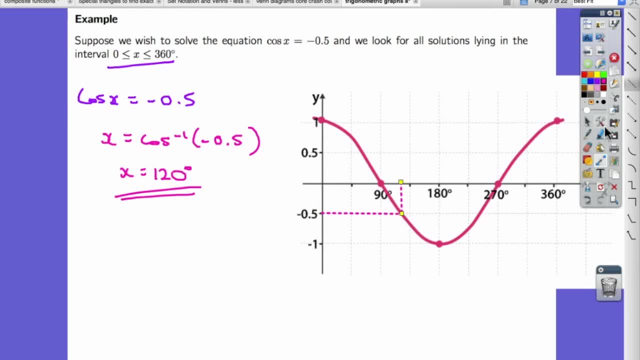 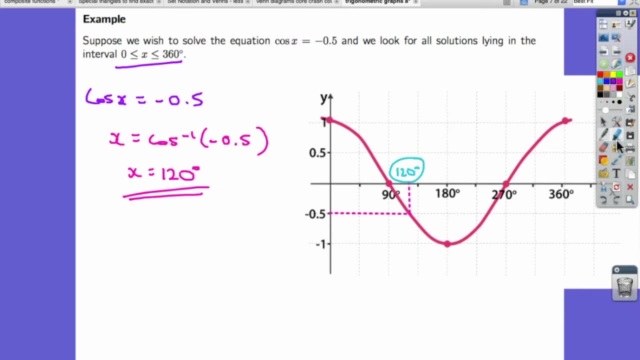 the graph and we're going to read up And, yes, it looks about right, It looks perfect to me actually. So 120 degrees is right here Now. then I'm going to do my sort of thinking again. Well, what I'll do before I do that is I'm going to extend that horizontal line. 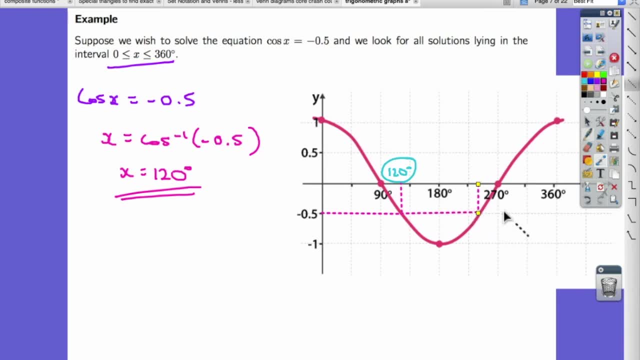 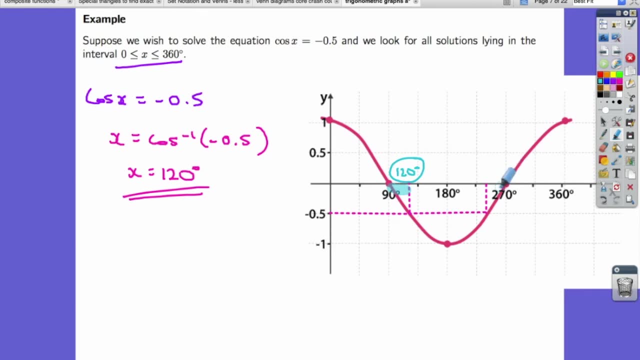 and check where we hit the graph again, which is just before 270.. Let's have a look at the difference between 90 and 120.. Again, it's 30, isn't it? So this, by symmetry, must be 30 as well. 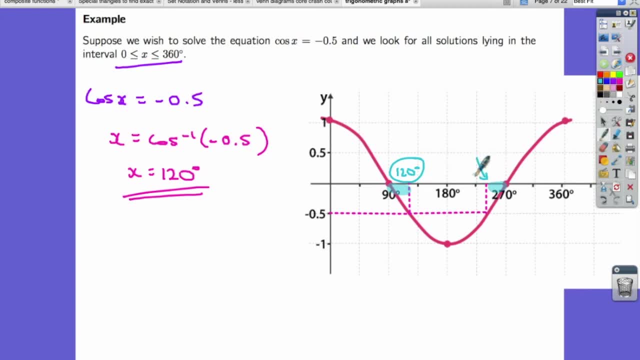 So I think that, and I hope you agree here, that the distance there, if that's 30, the blue distance here is 30. I ought to be doing 270 degrees Subtract the 30 degrees. that I know is that distance, to get this mystery value at this point, which is: 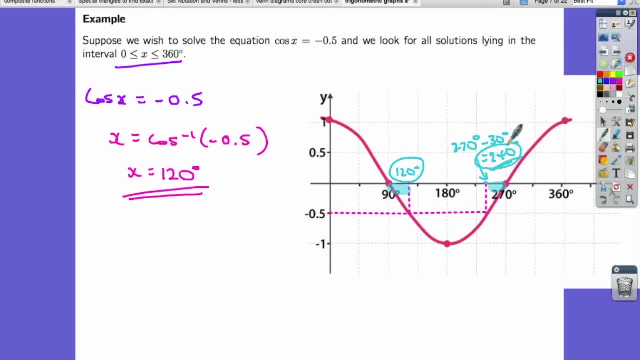 240 degrees. OK, and again, I can put that into my calculator and I can check it. So 240 degrees. I think that's my. they're my two answers. OK, so I'm going to go and check in my calculator that cos 240. 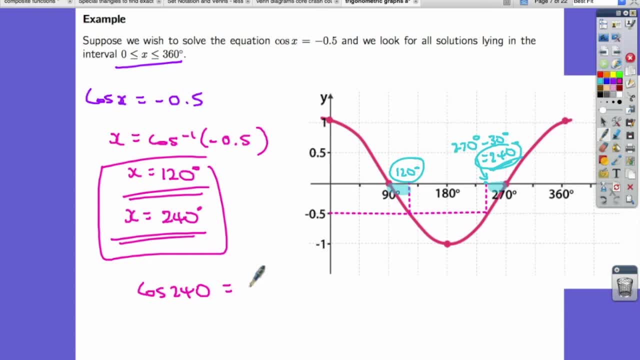 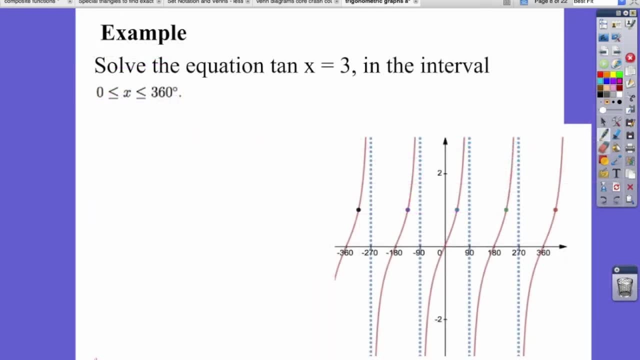 equals negative 0.5.. And I am absolutely correct there. OK, so great, I'm happy, All right. OK, final part. today, I'm going to show you how to solve an equation. I'm going to show you how to solve an equation. 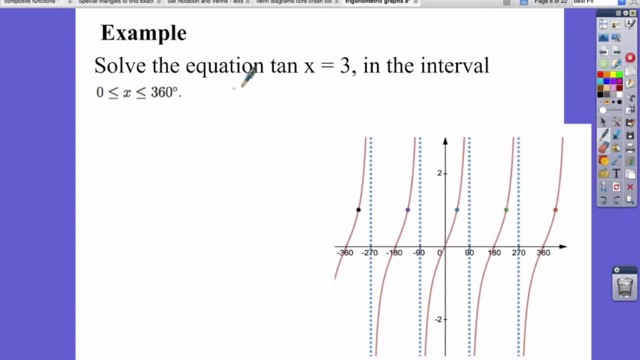 I'm going to show you how to solve an equation involving tan. OK, using the graph. So this one is: tan x equals three. They can see that the numbers gone up, because obviously the tan graph goes up infinitely. OK, its range is infinite in. 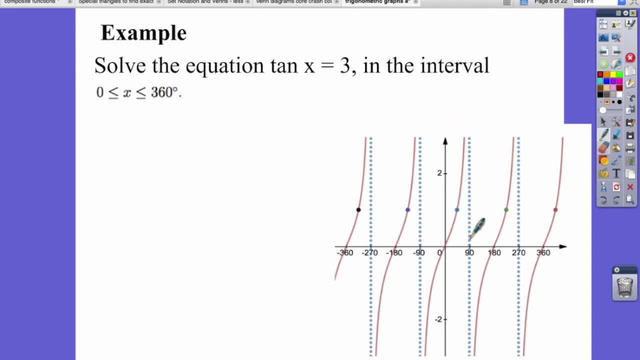 the vertical direction. It keeps going And, crucially though, it does have these asymptotes You can see at 90 and 270 and minus 90 and minus 270, which I didn't actually mention in my last video, But they're very important. We can't do tan. 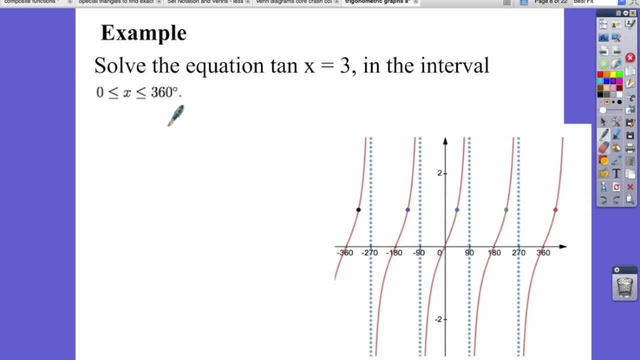 90. If you do that on your calculator You'll get maths error. And tan 270 doesn't work either. So we might come on to that reason for that in a later video. But here we go. So let's stick to the point. We've got tan x equals three And 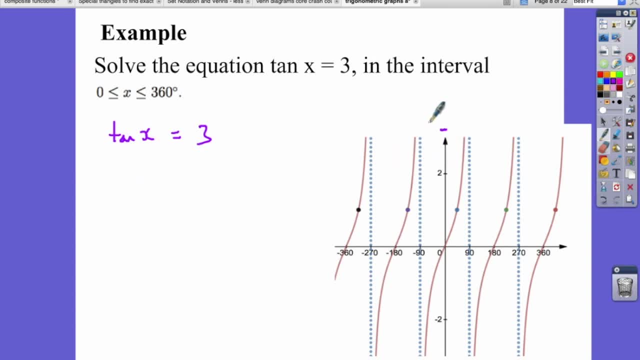 we can solve this because obviously you can see two, three will be up here somewhere. All right, We can go across the graph and read down. So it would be something just a bit less than 90, probably. OK, so the x is tan to the minus one of three, And if I put that into my calculator, 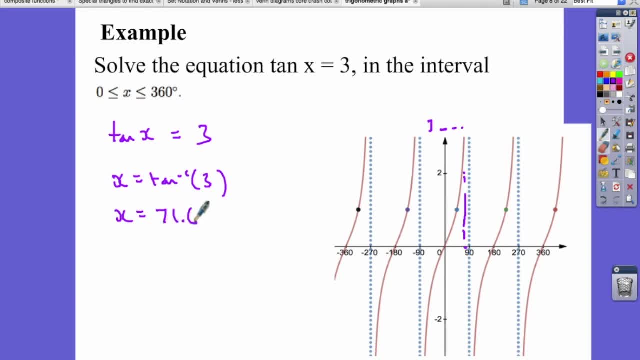 I get an answer of 71.. 0.6 degrees to one decimal place. Now, we talked in the last video as well about how this- the snakes, as I like to call them- they actually repeat themselves every 180 degrees. 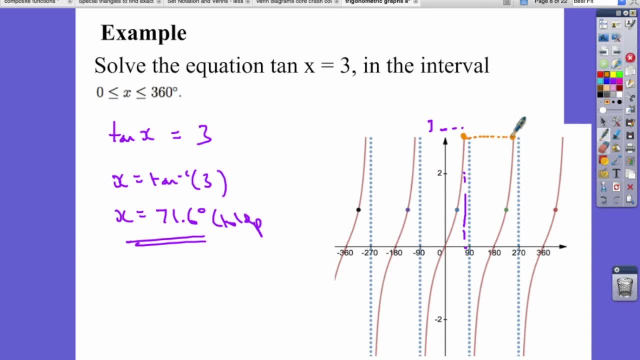 They say that my answer up here is there. OK, That is going to be repeated 180 degrees later. So all I need to do for this one is just add on 180 degrees to my answer to get the next answer along. um, so if I do that, I get 251.6 degrees to one decimal place- really easy with the time graph. 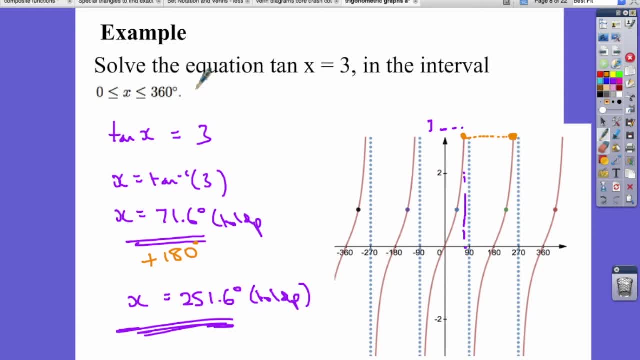 actually. okay, now I can go and check the next one and check it's still in the range. but you remember I'm in, sorry, the domain, the domain is zero to 360. so if I go across the next one it does actually become 431.6, which is too big. okay, it's outside of this, isn't it? I really want to go. 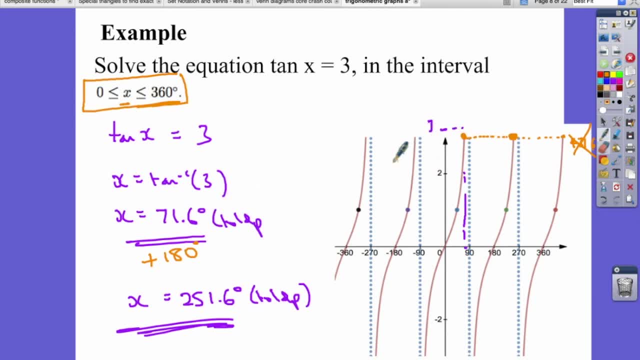 up to 360 and obviously going backwards I'm going to be going negative. so I've actually got my two answers there really easily just from adding on that that 180. all right, so I've got my first answer at the calculator and then I just added on 180 to get my second answer. easy as that. okay, so I hope. 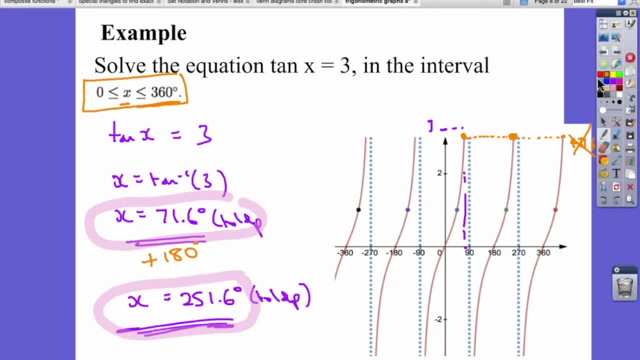 you enjoyed this video and if you did hit subscribe, go support my channel and keep enjoying my videos. thanks,